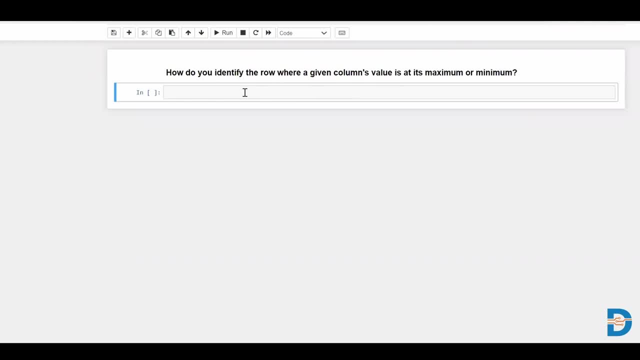 index number. So we have to find it out. So how do we do this? So first I'm going to import my pandas as pd, and quickly I'll import my numpy as np as well. Then I'll create one data frame. so I'll say df equals to pd, dot data frame, and then 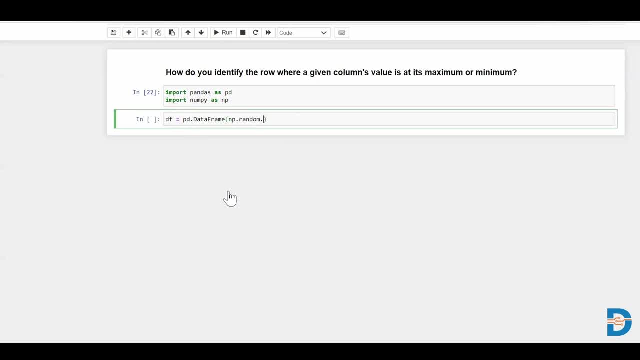 inside of it I'll say np, dot, random dot and I'll create like five by three matrix data frame, basically five rows and three columns. I'll say five comma three and then comma. then we have to specify the name of the column. so I'll say columns equals to a, b, then c. Let me run my df, I could see I have a, b, c columns. 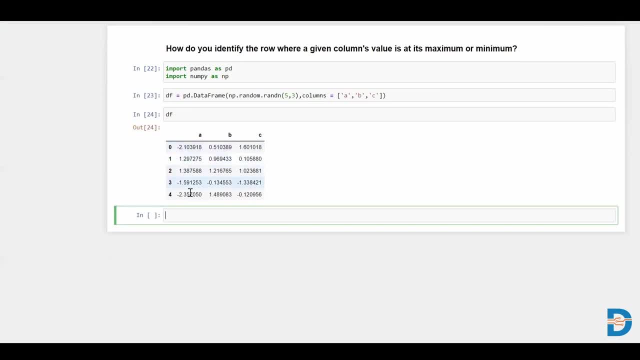 and this is a five plus three data frame. okay, So let's say I want to know what is the minimum value for the column a. So for that, first I'll select my a column and then I'll say dot min. When I run I get that: minus two, minus two, point three. five seven is the minimum value and I got. 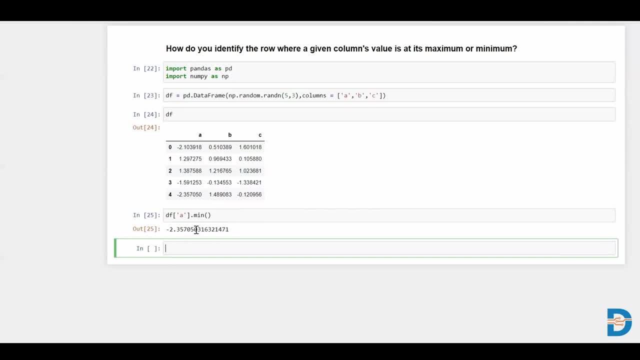 the minimum value like this. But let's say I want to know what is the corresponding index number. It's where the column a is having the minimum value. So for that I'll select my a column and we have a functionality called idx min and this idx min will say what is the 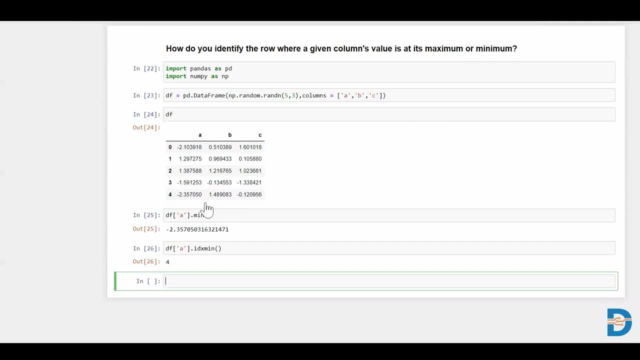 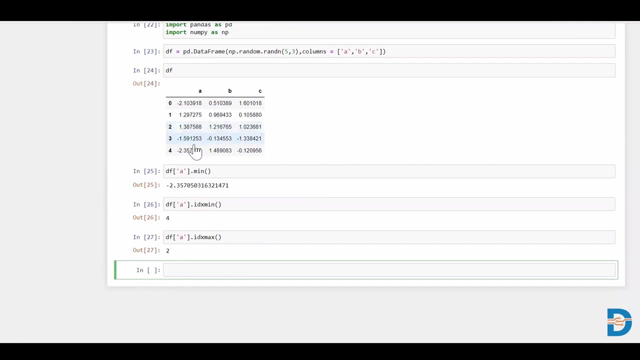 row index number for that particular minimum value that is existing in column a. okay, Similarly, if I say df of a, then idx max. I run this, I'll get two, because two is the index number where the column a is having the maximum value. that is nothing but one point. three, eight: